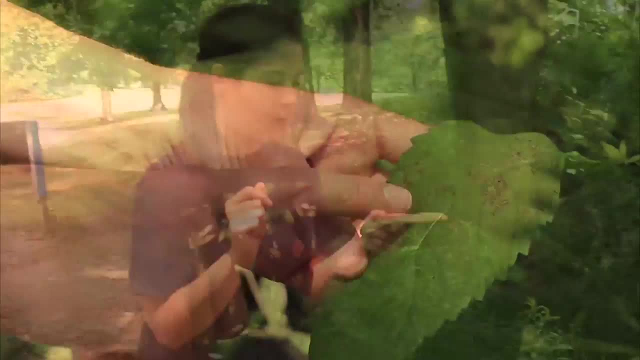 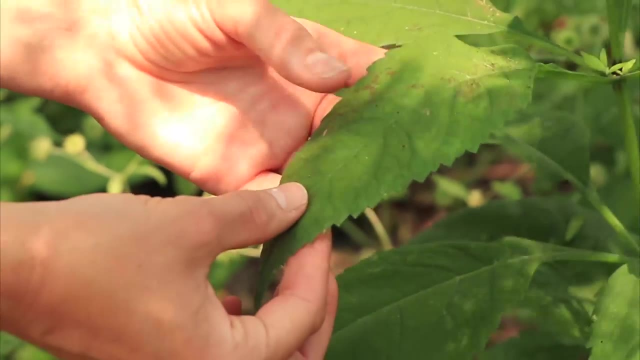 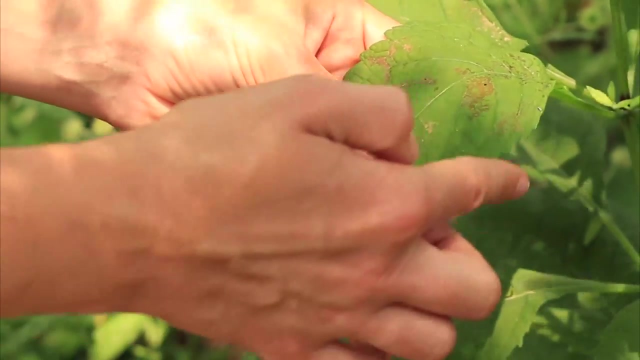 too. Let's see, Let's give this leaf a gentle touch. The top is really really quite soft, and now I wonder what this edge will feel like. Wow, All of these little V's on the margin. they feel kind of bumpy on my fingers. Really neat One. 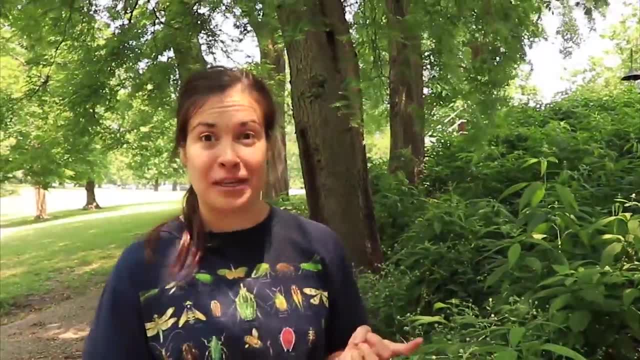 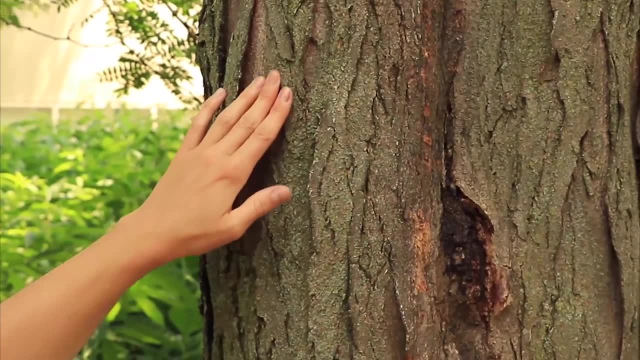 of my favorite things about plants is that they're really soft. They're really soft and they have really nice leaves and they feel quite kenny and soft. So what I'm going to do is I'm going to take this plant and I'm going to take 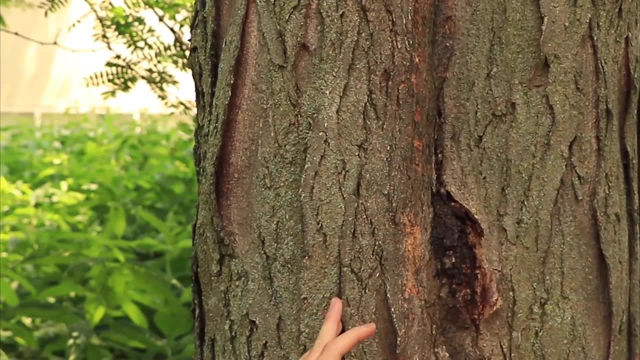 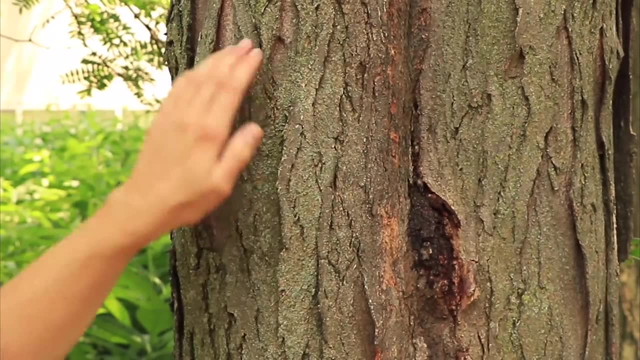 this piece of weed and I'm going to put it right here. I'm going to take this flower and I'm going to mix it with the thankiy I just put on the tree and I'm going to mix it with the plant and I'm going to put it. 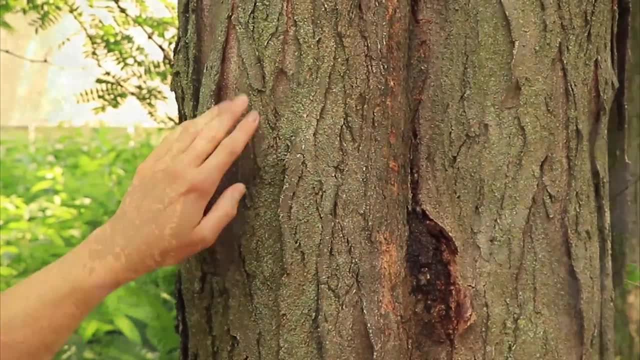 on my hand and I'm going to put my fingers on the tree and I'm going to press it and it's going to pop out, Oh, wow. so we can really feel all of the notes in this. for us to use our eyes for some good close looking. 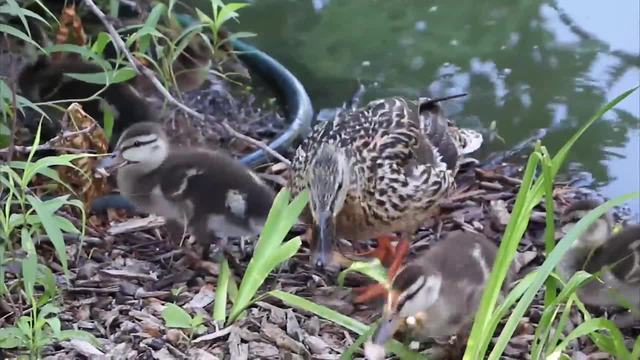 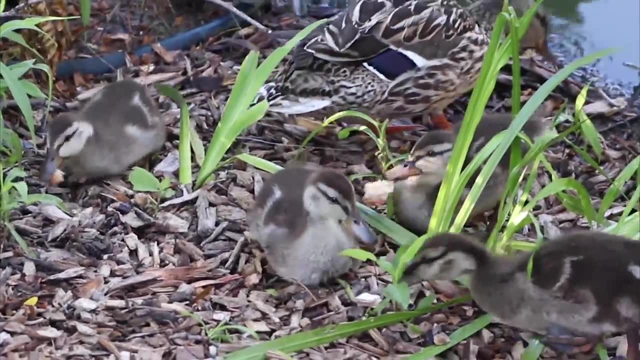 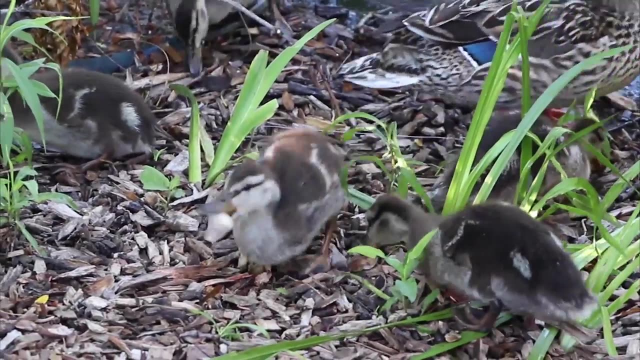 Let's check it out. right down here, I see something so interesting. Do you see it? Some ducks. What do you notice? Think about their color and their shape. What do you think they're doing? Yeah, I think they're eating too. 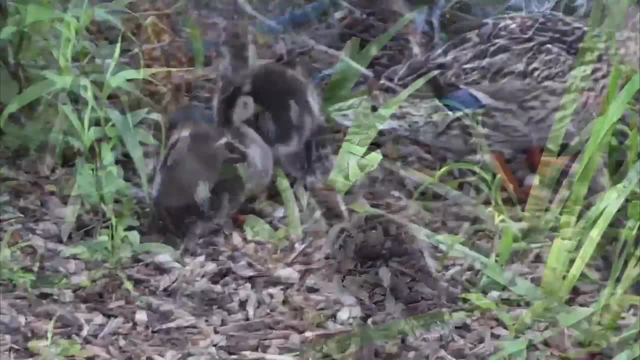 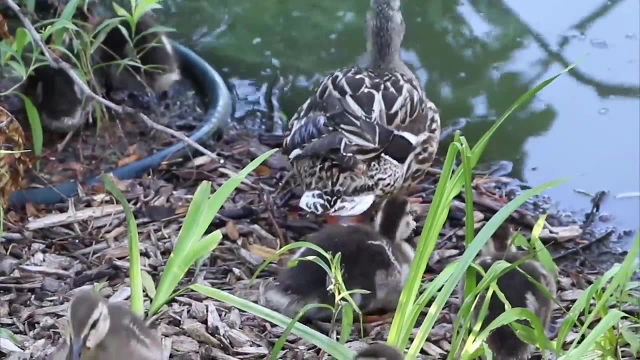 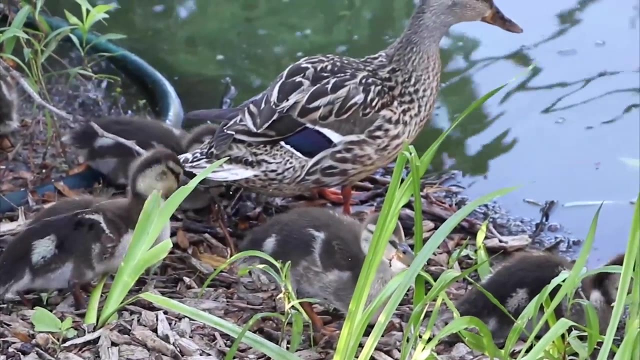 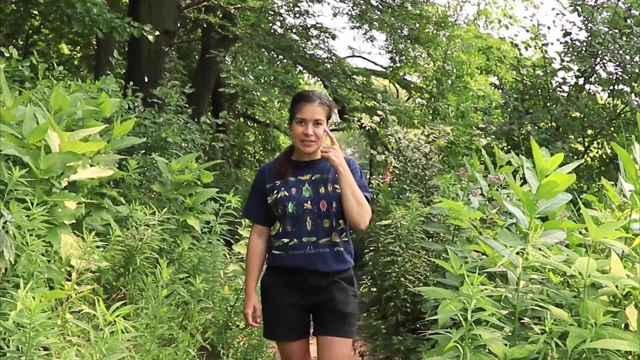 Oh, good eyes. Do you think all of these ducks are the same age? I don't think so either. How many of those baby ducks do you see? How big are they? This looks like another good spot to use our eyes. Oh, let's check out right over here. 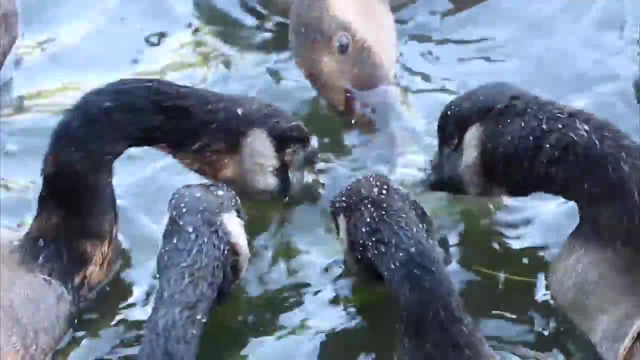 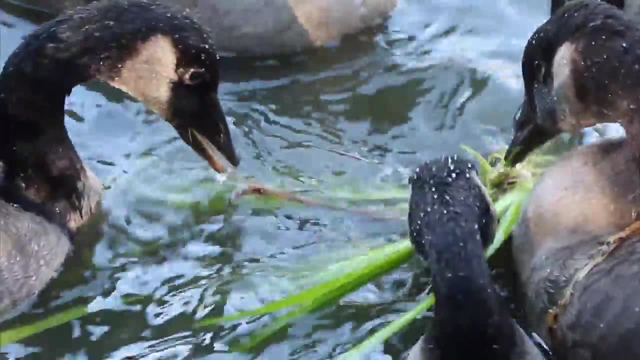 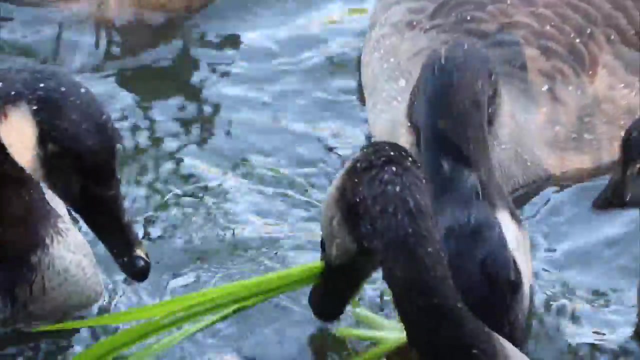 I think I see something interesting. Do you see it? Oh wow, Check it out. What do you notice these geese doing? Yeah, I think they're feeding. Really cool. How do the geese compare to the size of our duck friend? 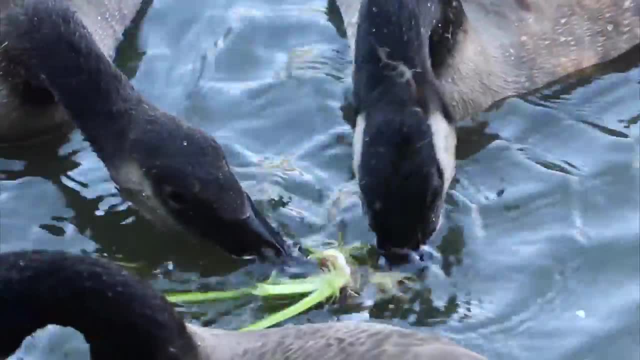 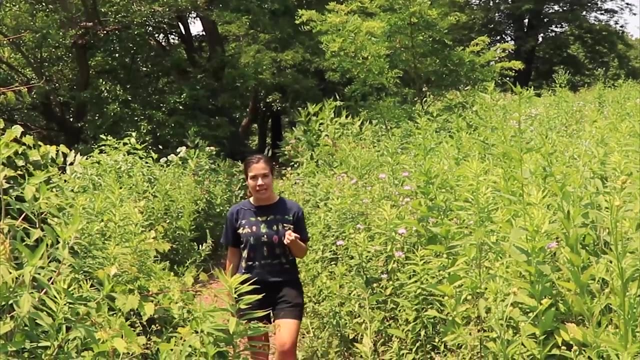 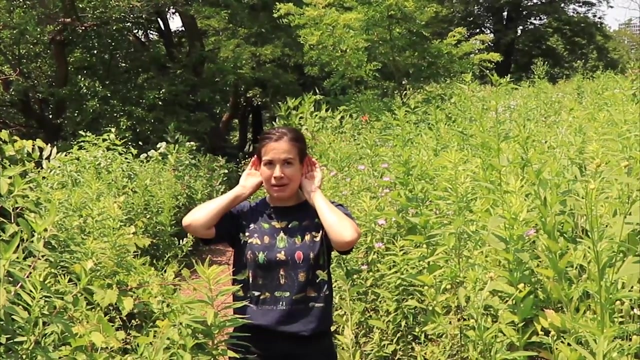 Yeah, they're a lot bigger. Excellent observation scientist. This looks like we can find a great place for listening right in here. I like to make my ears. I like to make my ears as big as I can by putting my hands behind them for listening. 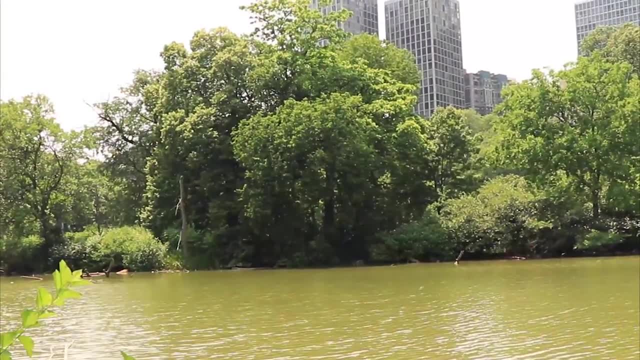 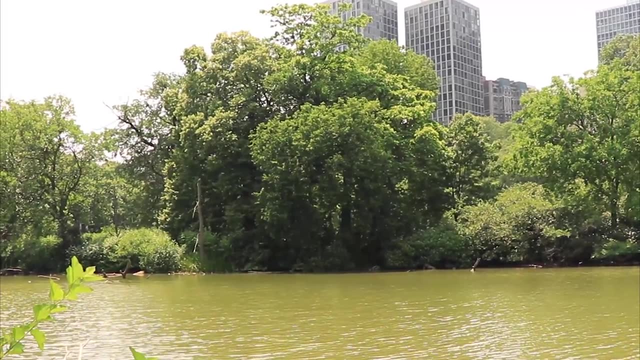 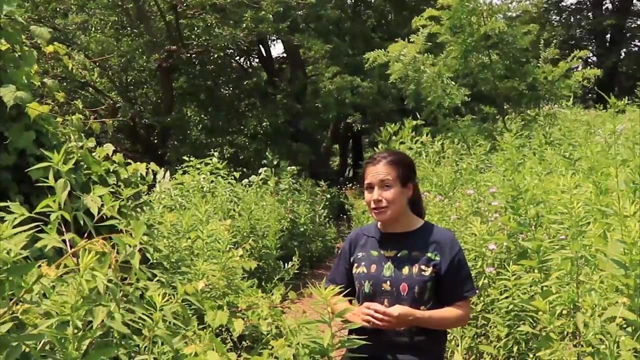 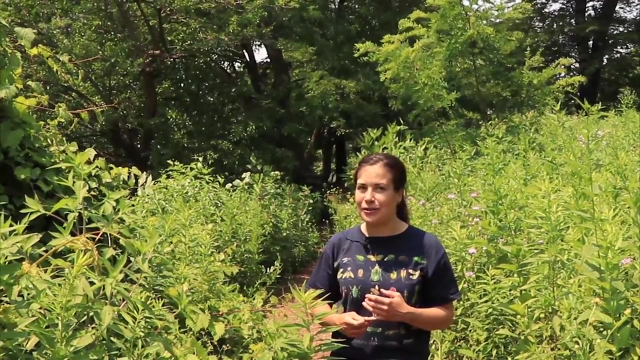 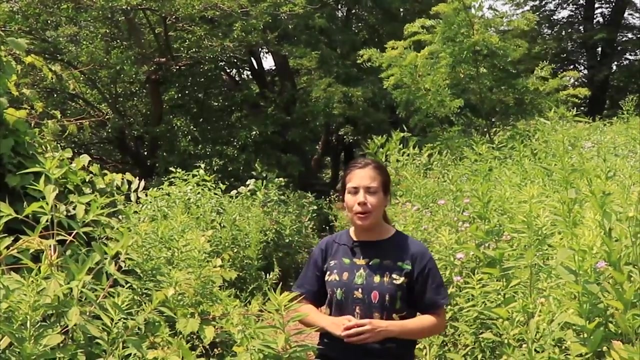 Let's see what we can hear. Wow, I heard some really interesting sounds in there. I definitely think I heard some bird sounds. Did you hear them? I think I also heard some human sounds too. I think I heard an airplane. I love focusing in on the nature sounds I hear. 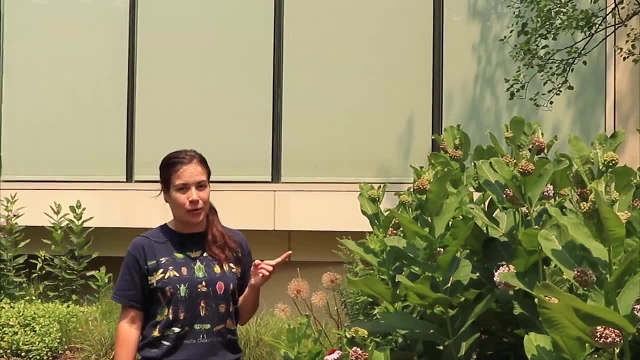 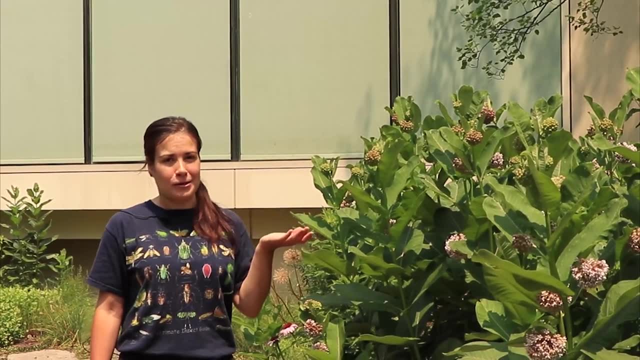 but we know we'll hear some human sounds too. This looks like a great place where we could use our sense of smell to smell some flowers- And we can often find flowers in parks right near your home, And smelling flowers is a wonderful way for us. 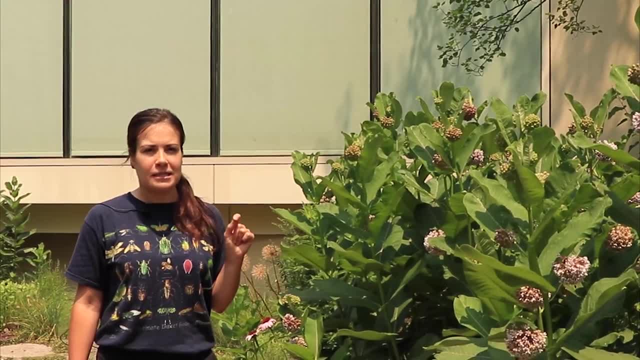 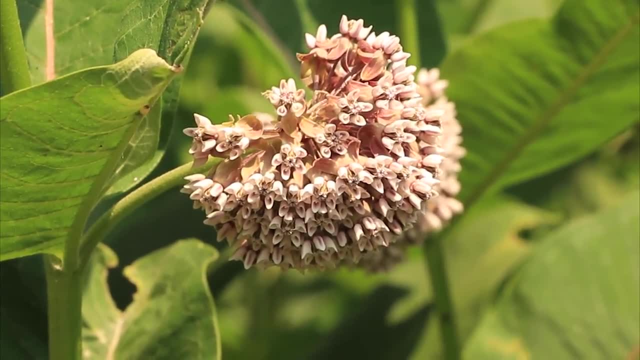 to use our senses to learn more about the plants around us. Let's stop and smell some flowers. Oh, let's give this milkweed a little smell. As long as we aren't sharing this flower with any insect, we can notice a nice, sweet smell. 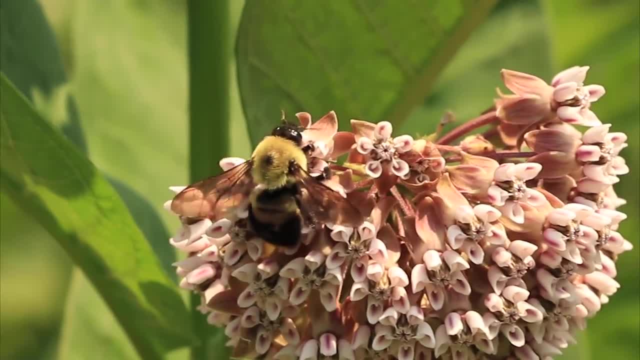 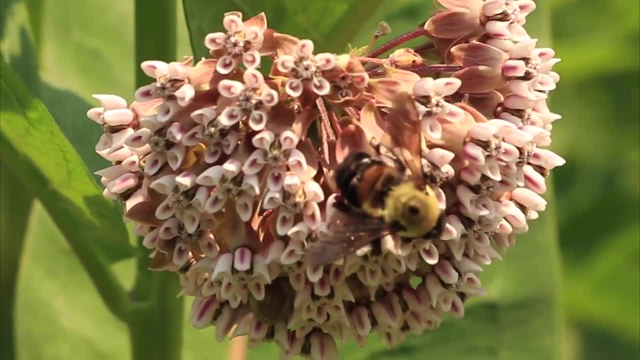 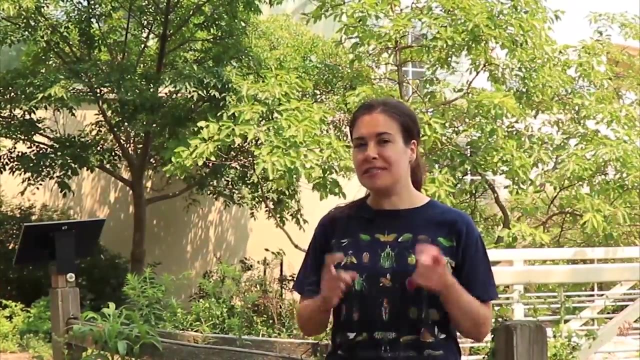 Really neat. I also notice lots and lots of insect friends who are also enjoying this flower for its sweet flower juice, nectar. Another great way to use our sense of smell when we're outdoors is just to take a nice deep breath and notice the smell of the air. 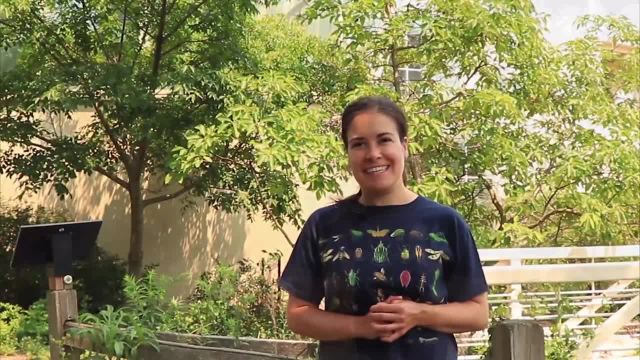 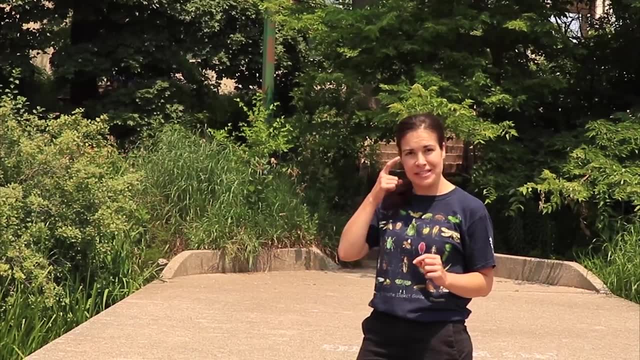 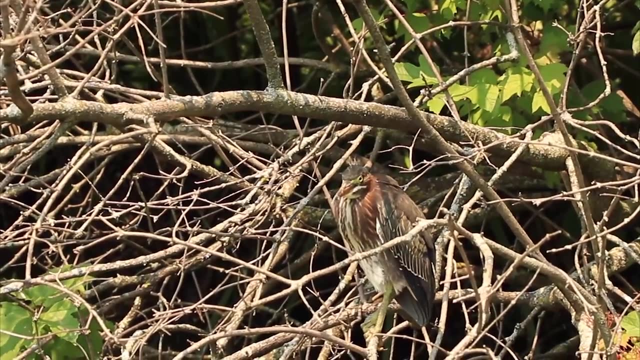 Ah, it smells nice. We're down close to North Pond And if you're near water, it's another wonderful place for you to use your eyes to explore. Wow, down there I see a small bird, Do you see it? 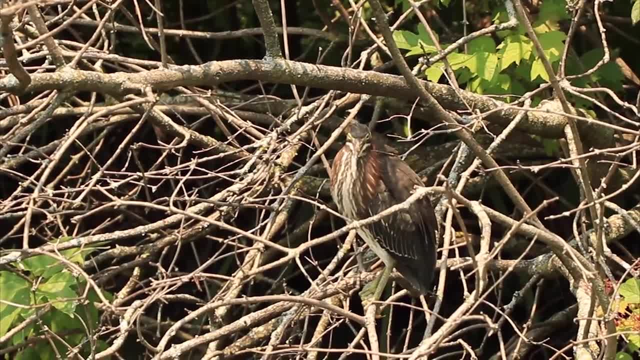 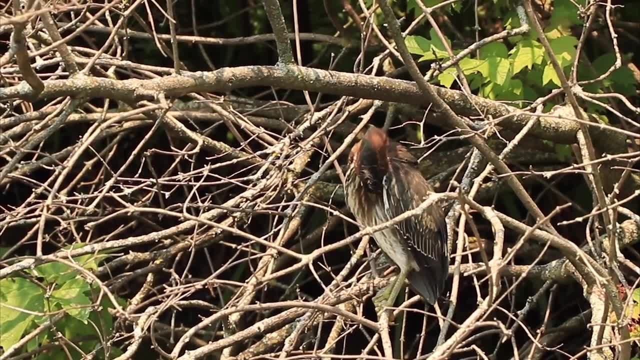 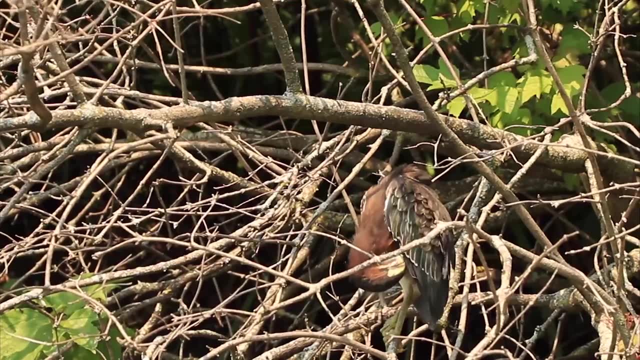 That is a small green heron. What do you think it's doing with its beak? Look at it, poking its beak Into its feathers and under its wings. What else do you notice about heron? Near the edge of the water is a great place.